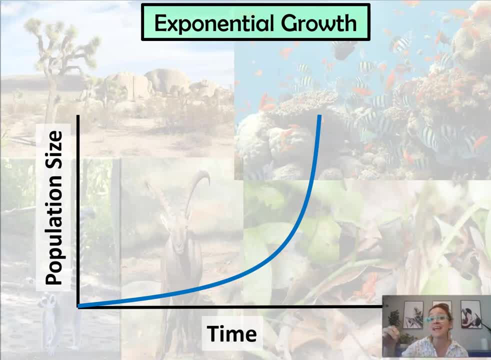 So what we just saw went from 1 to 2 to 4 to 8 to 16,, 32 to 64.. It's going to keep on doubling 128,, 256,, 512, and it's going to go through exponential rate of growth. 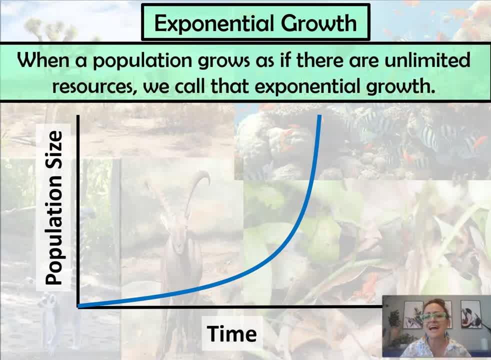 And in exponential growth the population grows as if there's unlimited resources. Now, in bacteria that could be. they could be growing exponentially within a petri dish until they run out of space Or run out of nutrients, But in reality a population you don't see exponential growth sustained for very long in nature. 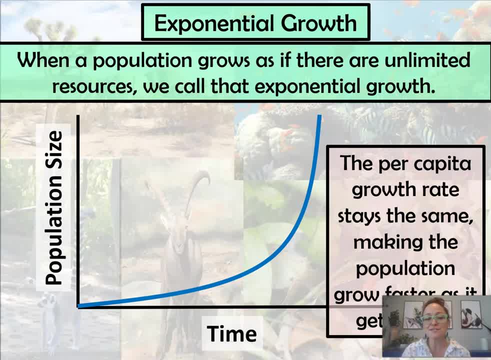 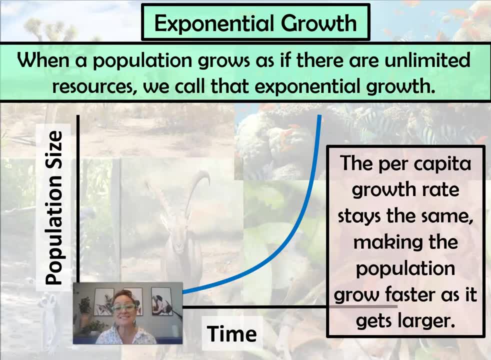 But let's still spend some time talking about it. So when we talk about exponential growth, the per capita or per individual growth rate stays the same. So in the bacteria it was doubling right Every 20 minutes, Like that rate of increase stayed the same. 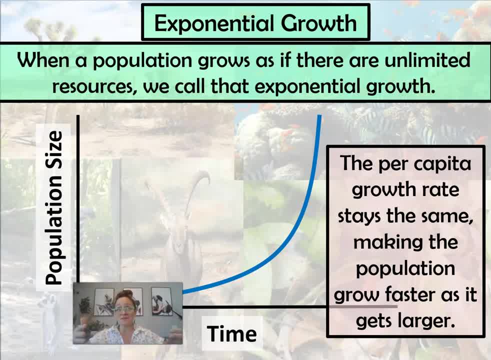 And therefore, as the population grows, it stays the same. And as the population got larger, it grew. I mean there's even more now doubling, And then all of those doubled, And so as the population gets larger, it grows faster and faster and faster. 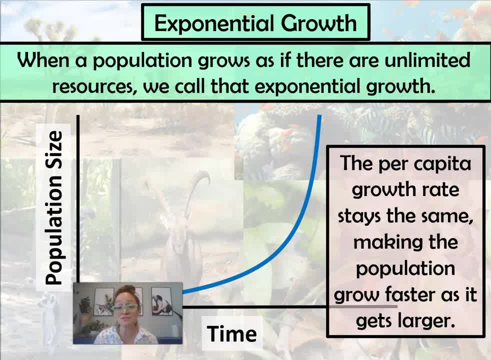 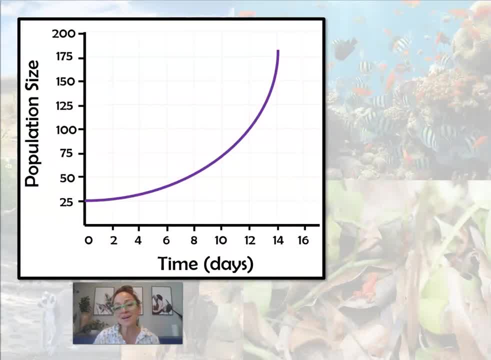 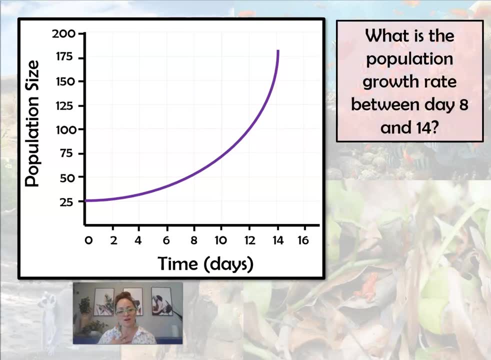 So humans have been experiencing exponential growth for a while now And our population is increasing like crazy All right. Now, when we talk about exponential growth, it ends up making what we call a J-shaped curve, And you may come across a couple different styles of like math problems or getting asked about population growth. 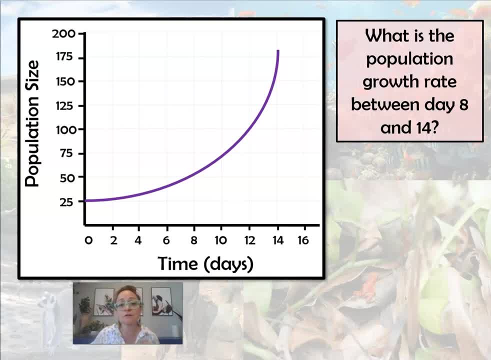 So in this one we're going to just look at, like, how do you calculate the growth rate of this population in a given time period? So in this we're specifying between day 8 and day 14.. So really, you're going to find what is your final population. 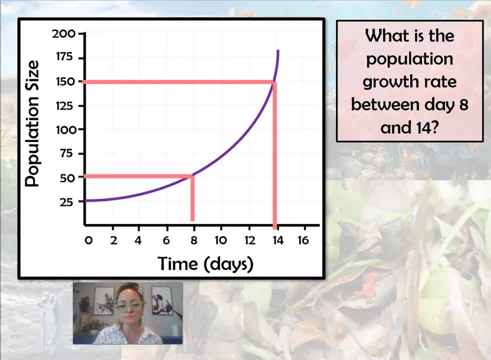 Here it was 150. And your initial population is 50. And now what we're going to do is we're going to find the final population And we're going to find the final population. So we're going to find the final minus the initial over or divided by the change in time. 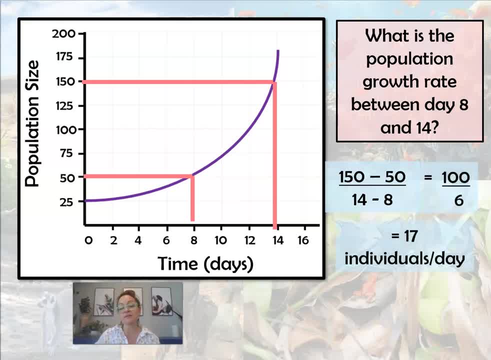 And so here we find that the average rate of growth was 17 individuals per day, was like, added to this population. And so if you ever have to calculate or find the rate of growth from a graph, you're going to want to find the final population size for whatever time frame they've mentioned, minus the initial divided by the change in time. 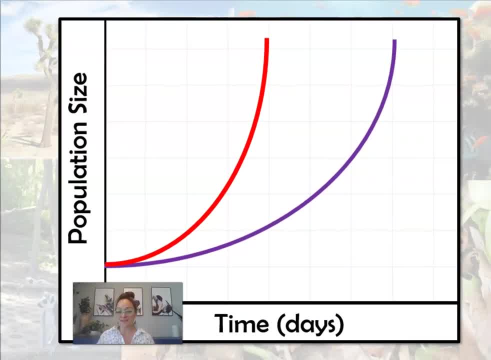 Okay, Good, Now something else you're probably going to see when talking about population growth rates is this value called R. Now, R stands for rate of growth And there's different ways to phrase it, But basically R is growth rate. 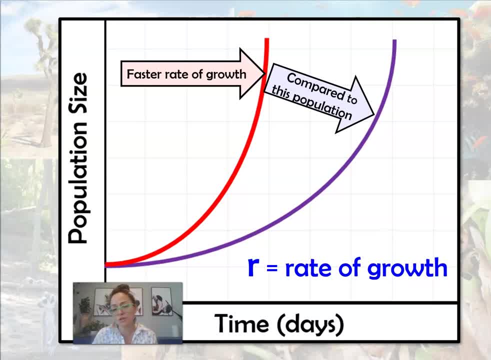 And out of these two populations we can look at the slope of the line And we can like envision that the red line is. this red population is growing at a faster rate compared to the purple population. So if I were to assign R values, 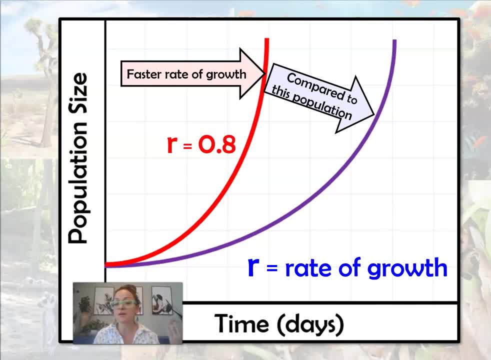 These are arbitrary. I made them up, But the red line would have a higher rate of growth compared to the purple line, So it's growing at a faster rate And therefore it has a higher R. Okay, So let's go ahead, though, and talk about some of the formulas you may see from College Board. 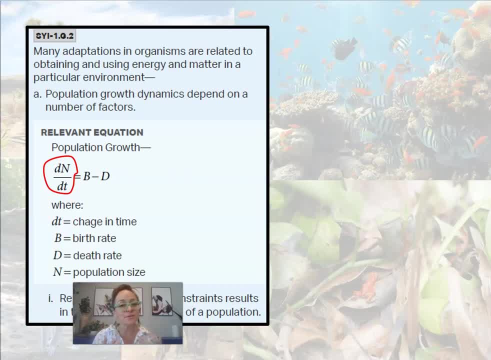 Now, when we look at these letters, a capital N stands for the population size And capital B is birth rate, Capital D is death rate, And so this is like per capita Or per individual in a population, And so like just realistically, when we think about birth rate and death rate. 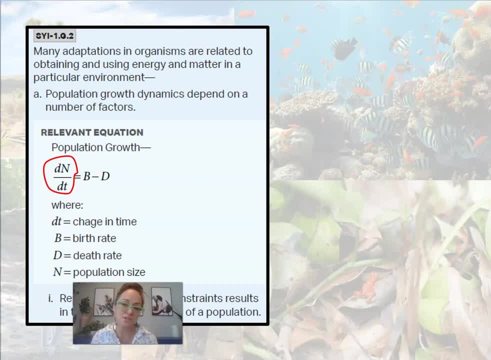 If we have more births than deaths, our population is getting larger. If we have more deaths than births, our population is getting smaller. Now, this area that I've circled here is kind of like like uses, not kind of. 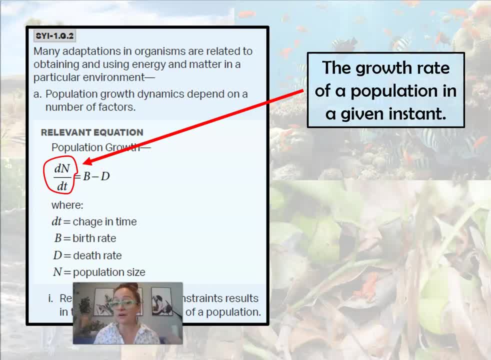 It uses notations that you would use in like a calculus class. But really that DN over DT is really like talking about how is the population changing over time, Like how is it growing, What is its growth rate? 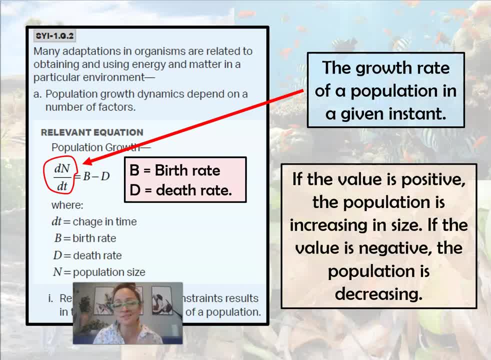 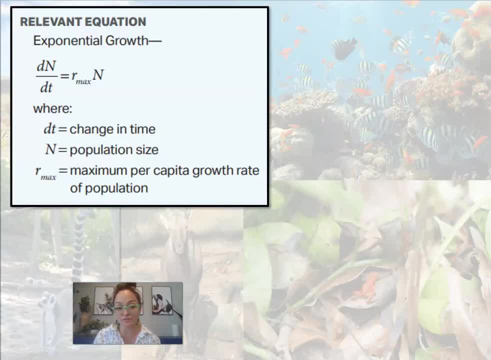 And so here I just want- this is words for what I just said. But if a population is increasing in size, you'll have a positive growth rate. If it's decreasing in size, you'll have a negative growth rate. Now let's go ahead, though, and look at the formula for exponential growth. 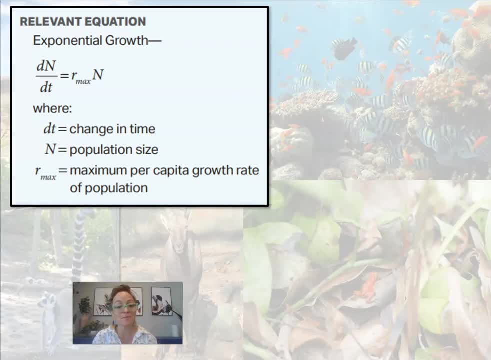 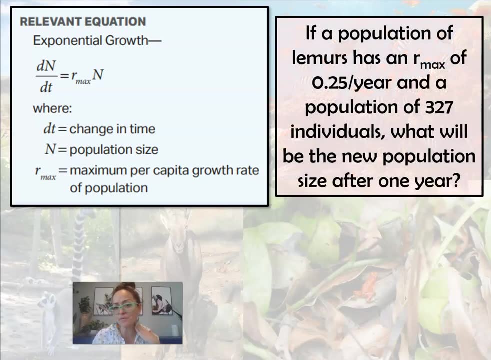 So we see R max. That's the maximum per capita growth rate. R max is the growth rate of a population, So that's per capita just means like per individual. And so here, if a population of lemurs has an R max of 0.25 per year, 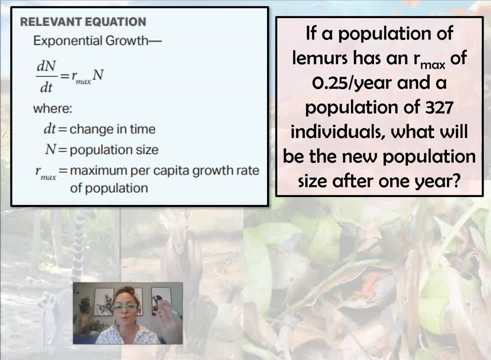 Now that 0.25 already takes into account the births and the deaths Like, this is our overall average rate of increase for this population. So it has an R max of 0.25 and a population of 327 individuals. 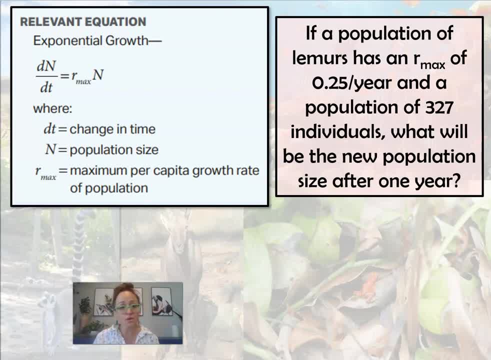 What will be the new population size After one year? Okay, So we take our formula And our R max is 0.25. And N is our population size And we find that the change in the one year like it was only one year. 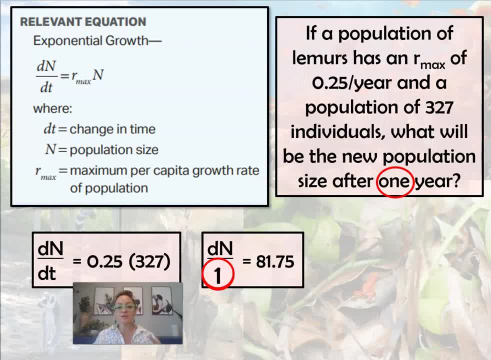 So our denominator is a one So really like our change in our population has basically increased by 82 individuals. So in that year there were births and there were deaths, But we had a surplus or an additional 82.. 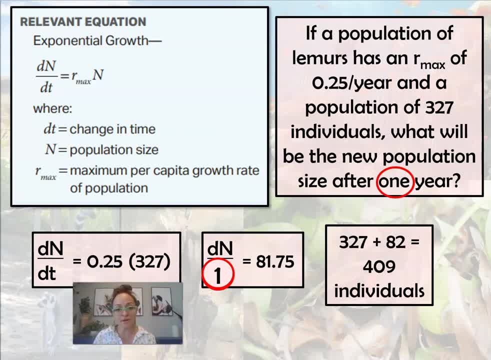 So we had a surplus, or an additional 82 individuals by the end of the year. So I'm going to take my 327 original population size And I'm going to add 82 individuals. So now the new population size after one year is 409.. 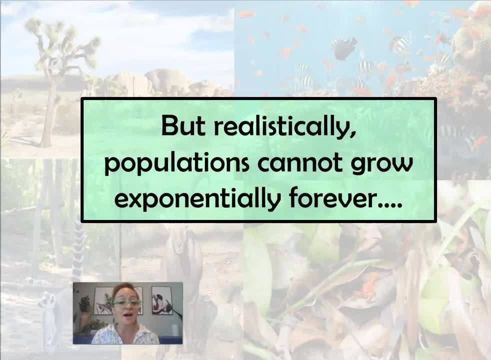 Now, realistically, though, populations cannot grow exponentially forever. There is going to be limited resources. Like you can think of Earth as, like an island: There's only so much land, There's only so many nutrients, Like, if you think about, like the law of conservation of matter. 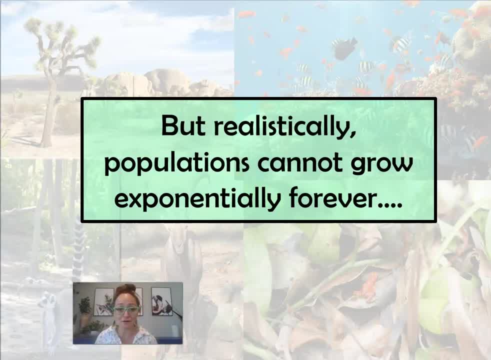 And like there's a limited or finite amount of resources on Earth, And so us humans, populations like as we, as humans especially, undergo exponential growth, there's going to be a point where we're running out of food, of space, of water. 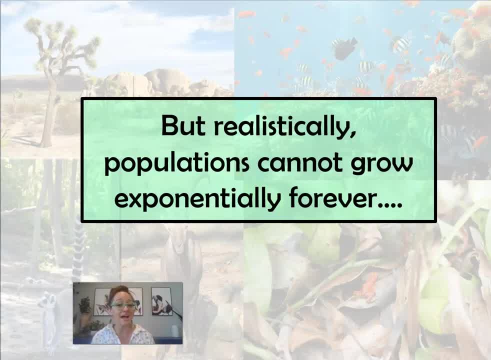 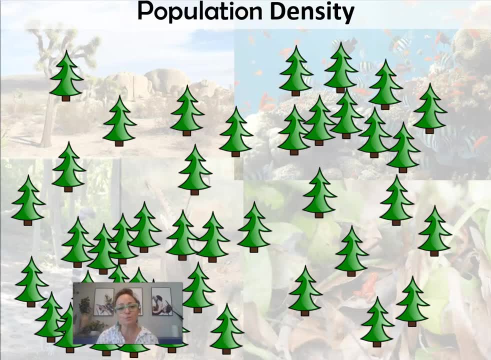 And then what's going to happen? Now, some would argue that's already happening in some parts of our world. Okay, So let's go ahead, though, and first talk about population density, so we can understand what happens. How does a population density increases? 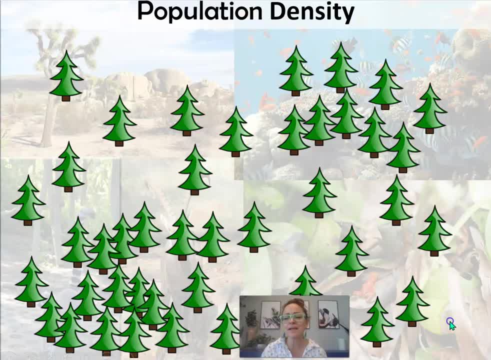 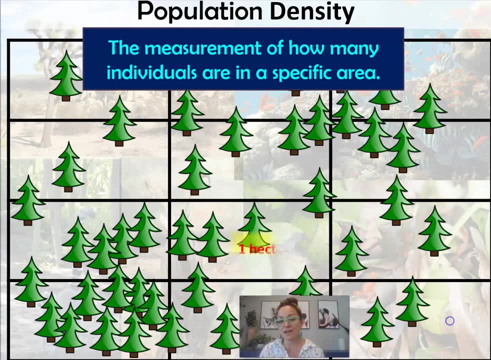 So here I have a forest, Let me move my face, And if I apply a grid to this forest, I can kind of measure, like, the population density in a specific area. So in this grid, though, because these trees are in a random dispersal pattern, it's not. 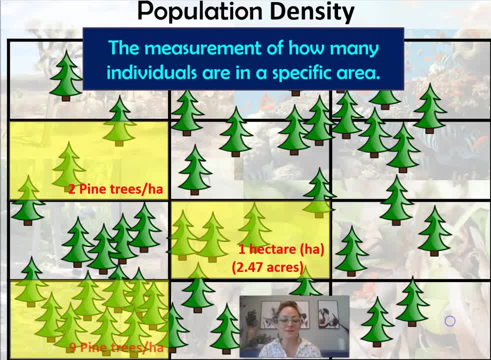 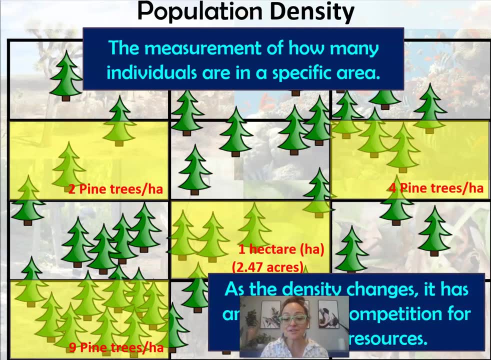 super, like even throughout the population, but like in this bottom left grid or quadrant, we would find nine trees per hectare, So that would have the highest density out of these three options. Now, when we talk, though, about populations as their density changes, so like how many? 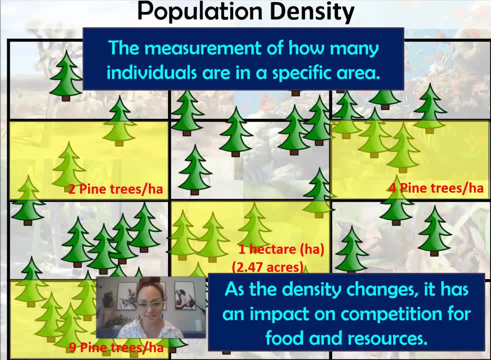 individuals are in a given area determines its density. So, for example, I teach in California and my average class size is about 40 to 42 students. Now that would be, 40 students in one classroom is a high population density compared to another. 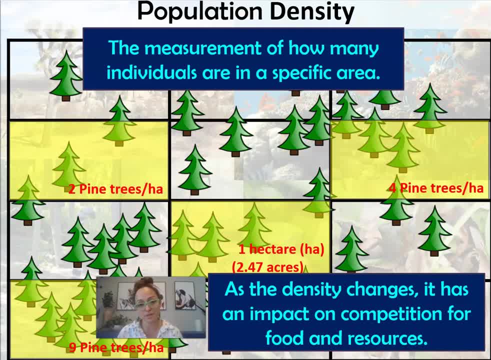 classroom So I have only 20 students. that would have a lower population density And as density changes it has an impact on competition for food and resources. So we can totally picture this that as you increase the individuals within a population, if they're all still in that same area, interacting together, they're going to have a more intense. 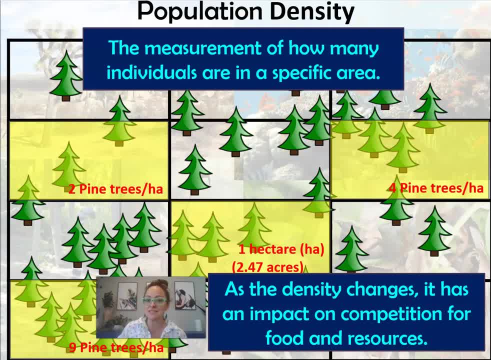 competition, that's going to get harder and harder to get all of the things necessary for life: Shelter, Water- I was going to say comfort, That's not one- But space right. So that is. as your population increases, it gets more and more difficult to have access. 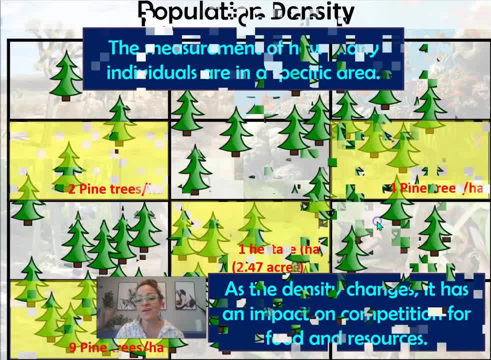 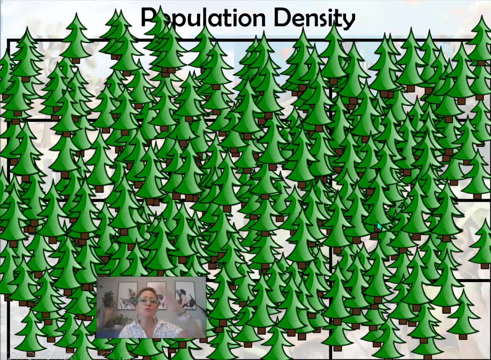 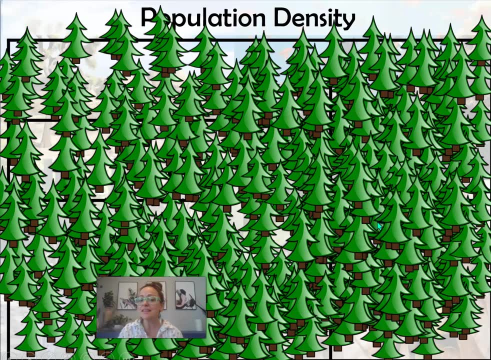 to all of the requirements for life, And so we cannot grow exponentially forever. If you think about this forest, if every seed that was ever dropped sprouted and grew to a mature tree, there would be intense competition for root space, for sunlight, for water, for 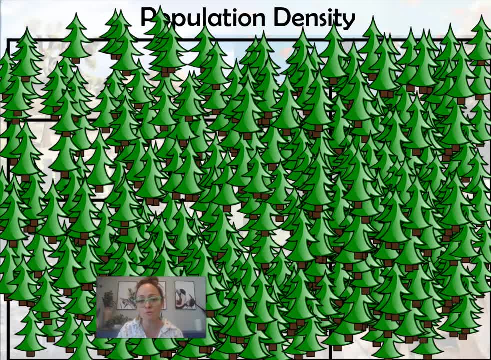 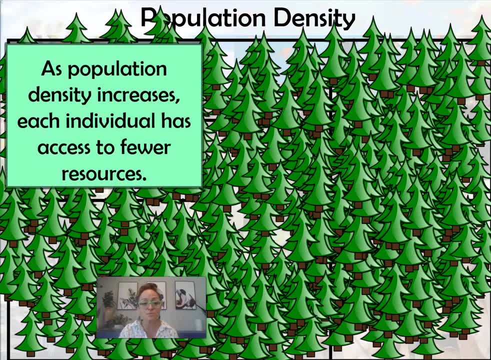 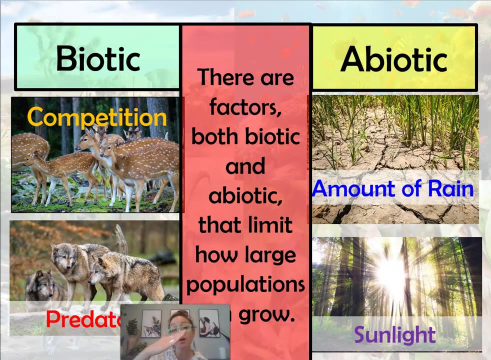 nutrients, And so the forest tree population could not grow on, grow on, go on increasing at a constant rate forever. It's just too many individuals, And as this population density increases, each individual has access to fewer resources. Okay, So if we think about what happens as populations grow and grow and grow, you're going to get. 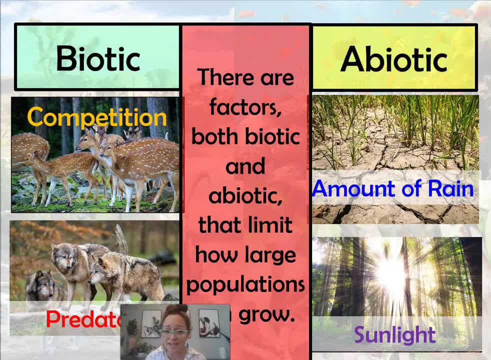 way more intense competition between individuals of the same population, And that's not good And that's going to lead to natural selection as well. But you also have predators. As your population increases, it makes it easier for predators to find you, And then we have abiotic factors that can influence a population size. 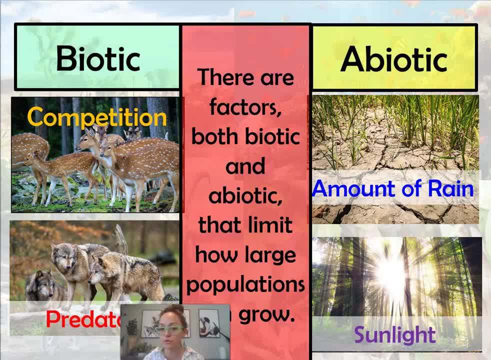 So you have things like available water, or are there enough nutrients in the soil, Or is there enough sunlight to produce enough food to support the food web or the population in that area. Okay, So there are a number of factors that can influence how large a population can grow. 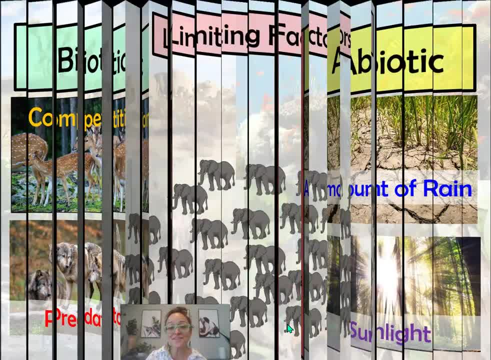 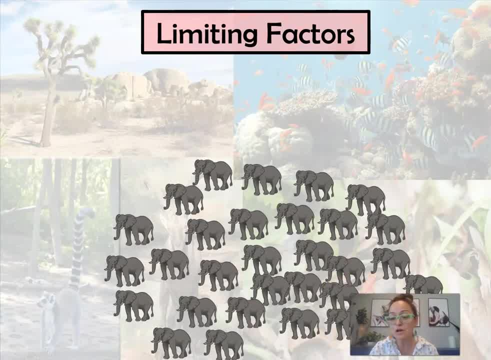 So darn okay. So when we talk about this, these factors that limit how big a population can grow are called limiting factors. So let's say we have a population of elephants here And there's reasons why these elephant population would not grow exponentially. 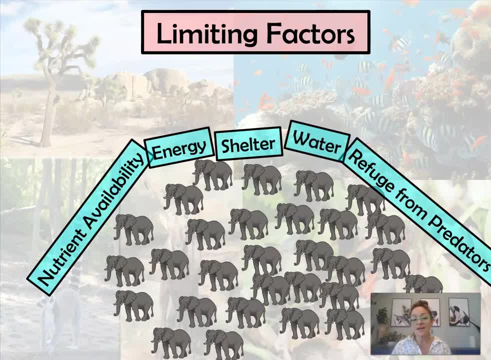 So it could be nutrient availability in the food that they eat. Okay, It could be the amount of energy. how much food is actually growing in their area, Because they're herbivores. is there enough plants to give enough calories to support the whole population? 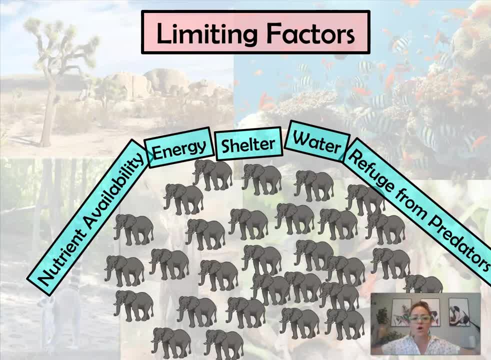 Shelter, water, refuge from predators- all of these things are factors that limit how big a population can grow. And if a population starts to multiply, they give births, the population increases in size. these limiting factors limit how big a population can grow. 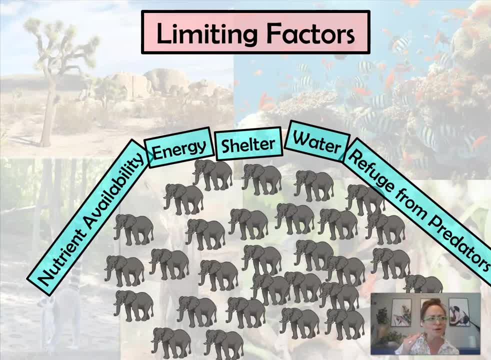 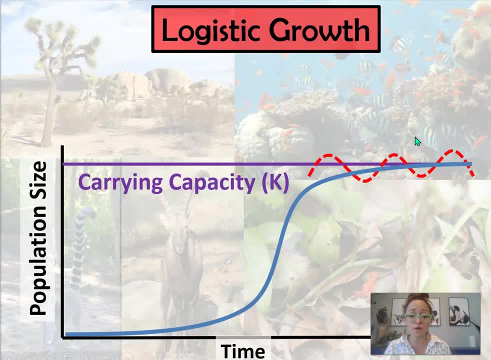 How big a population can increase, And so you're going to have births, but you're also going to have deaths, And so how those balance out really impact the population growth. And so if we look at- there's an area on a graph, though- 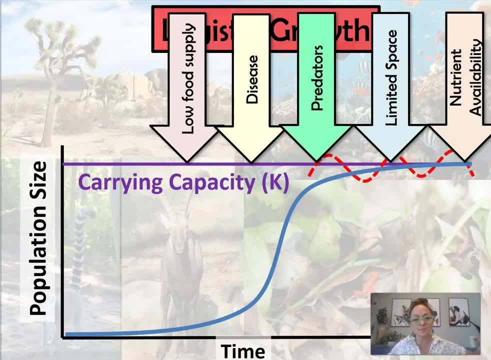 So here a population may undergo exponential growth. sorry, I hit pause. I think I was saying: as a population undergoes exponential growth, it starts to like feel the effects of what we call density dependent limiting factors. So maybe low food supply, more intense competition, limited space. 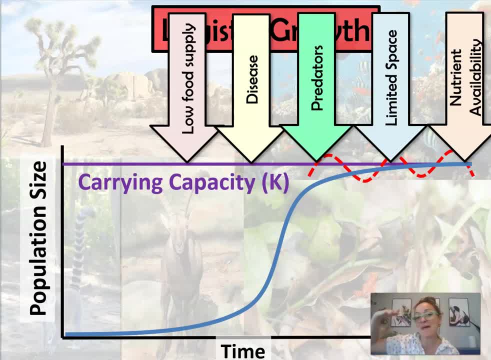 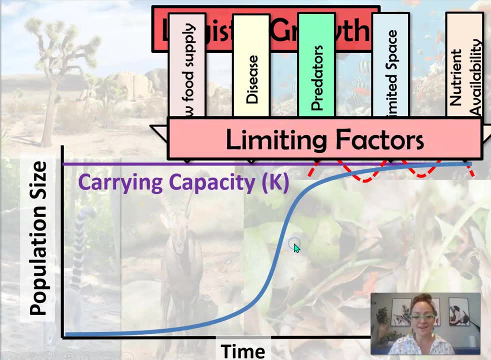 And so, therefore, the population reaches its maximum capacity for an area. So we call that the carrying capacity. The carrying capacity is like the max number of individuals that an environment can support of a particular population, And so let's go ahead and oops. 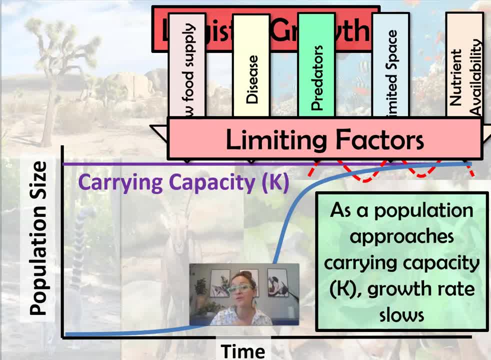 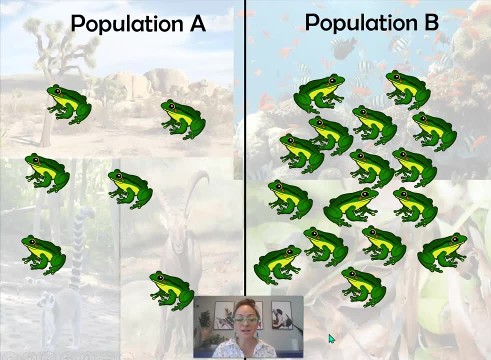 So, as a population approaches carrying capacity, though, the growth rate slows, And I'll talk about that and show a couple examples in a bit. So let's go ahead though, okay, And see some of these limiting factors that exist in nature. So we have two populations here, and you can see that population A has a lower population. 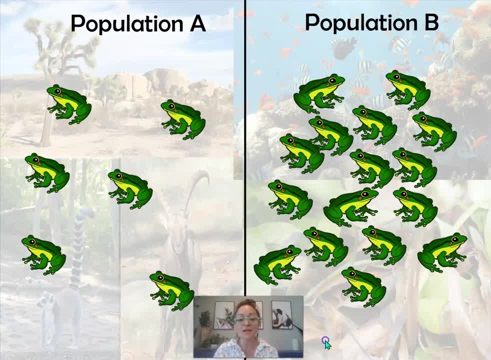 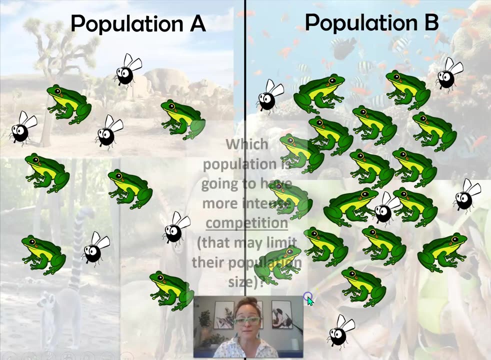 density and B has a higher population density. So when we think about food or food availability Or like Energy availability, we want to ask ourselves which population is going to feel the effects of a limited food supply. It's going to be population B, right? 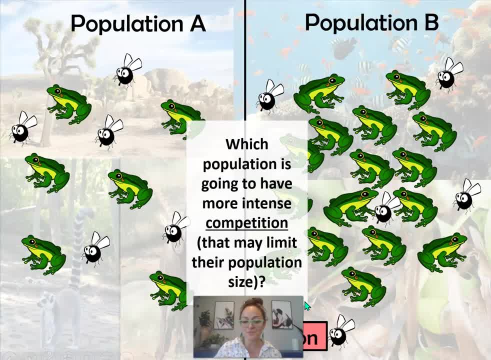 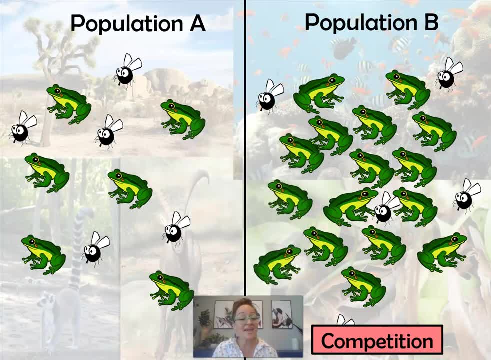 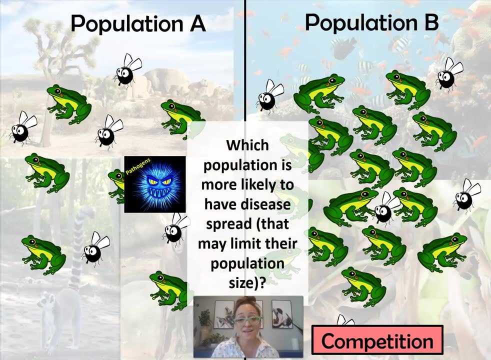 So population B is going to have pretty intense competition for resources. Competition is a limiting factor. It's going to limit who's able to survive and, based on the amount of food that they were able to access Now, which population is more likely to have disease spread. 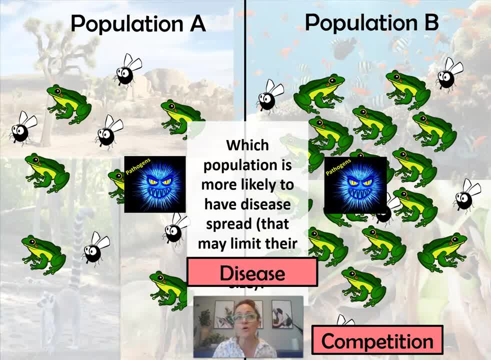 That's also going to be population B. Think about, like With COVID, for example, we had the social distancing, the spacing of six feet, like the more spread out we are, the less likely the disease will spread. Same thing in populations. 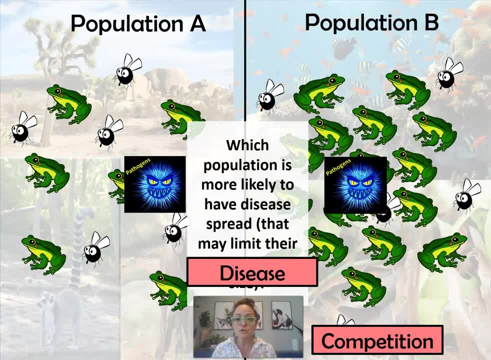 Disease is spread through natural populations in the wild. So the higher population density, the easier disease will spread and limit how big your population can grow. So disease is really going to have a greater impact the greater the density of the population. Okay, 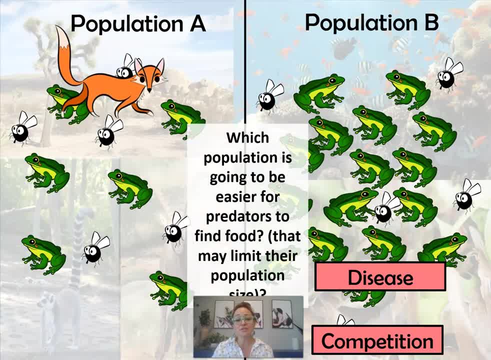 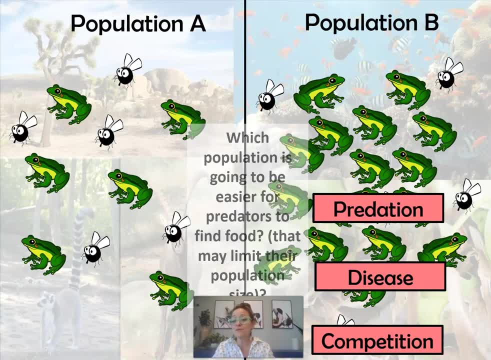 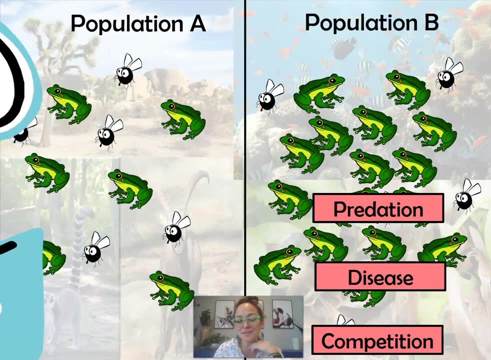 And then when we talk about predators and which population is going to feel the effect of predators, it's really going to be population B. There's going to be more prey available for the predators. So here now, if there's like a tsunami, though, or something, does density really matter? on, 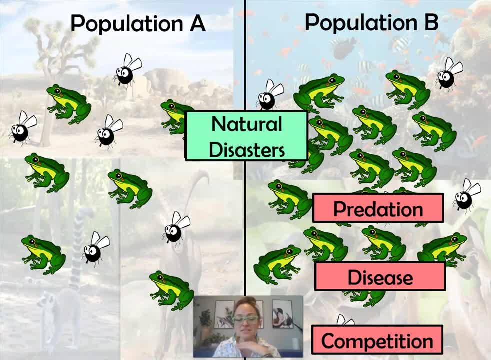 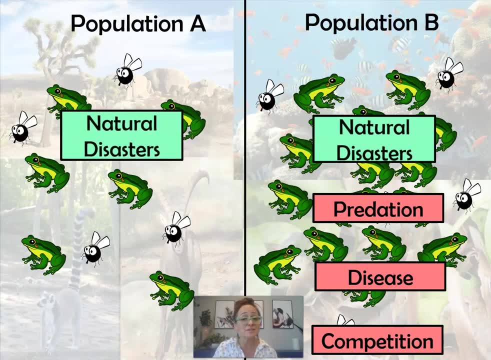 how the populations are impacted. Not really. Natural disasters don't really have anything to do with the density of a population, They're just a fluke thing, unfortunate thing that happens And it will affect both. Same with pollution, Pollution in an environment, whether it's air, water, noise, light pollution. they're. 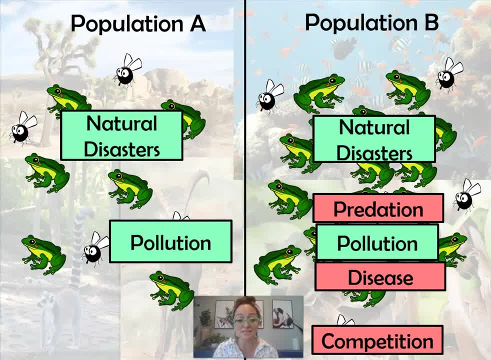 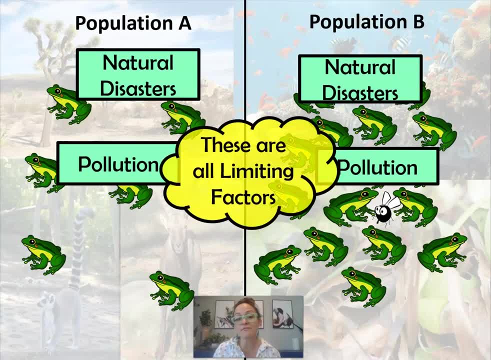 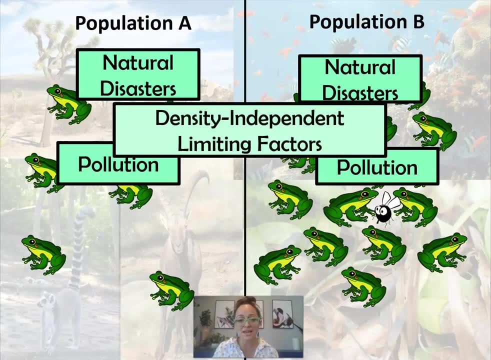 going to impact populations regardless of the population density. So when we look at limiting factors, we can divide them into two categories. Here we have limiting factors that are density independent. They're going to have an impact on the population size regardless of the population density. 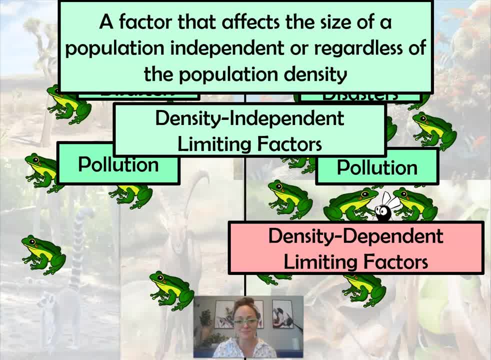 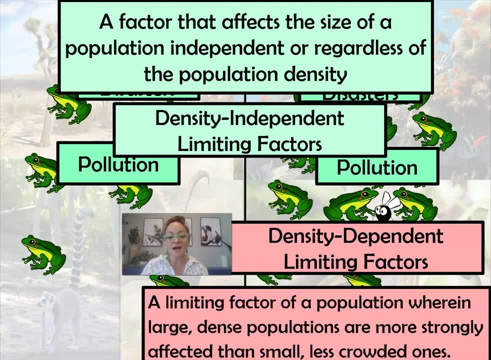 Okay. And then we have ones that are density dependent. So that would be your competition, your predators, your disease. Those are all limiting factors that large, dense populations are more strongly affected by compared to small, less crowded populations. So limiting factors really limit how big a population can grow. 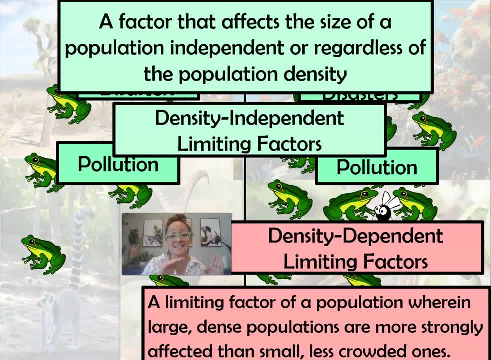 And they're divided into two categories: density independent and density dependent. Okay, So let's go ahead, though, and go back to logistic growth and talk about- oh, there's the words behind it. So your density independent? oh, okay, predation, disease, competition, okay. 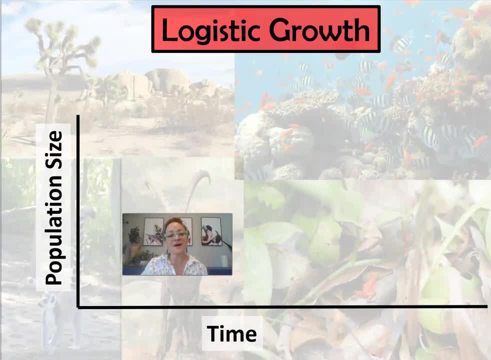 So let's go ahead, though, and talk about this graph, So when we talk about a real life example of logistic growth. so the elephants in a certain region in Africa were hunted to almost extinction in the 1600, the 1960s- sorry. 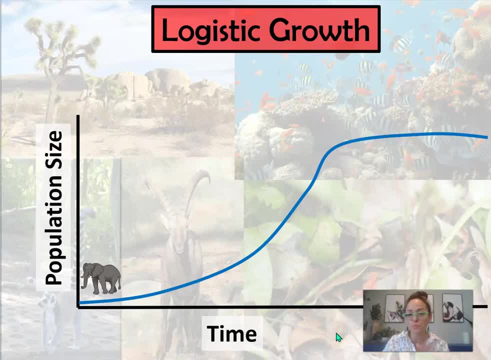 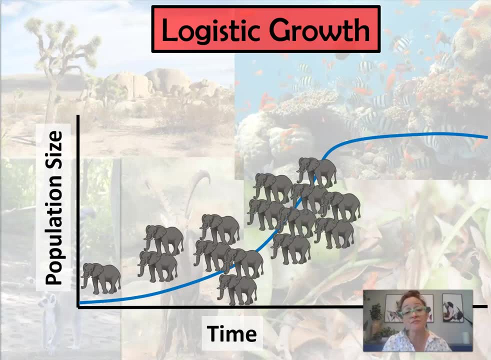 for their ivory tusks. Okay, So some rules were put into place to stop poaching, And what they found was that the population underwent exponential growth as they recovered over the decades. So they had- it was as if there were unlimited resources, but eventually their population. 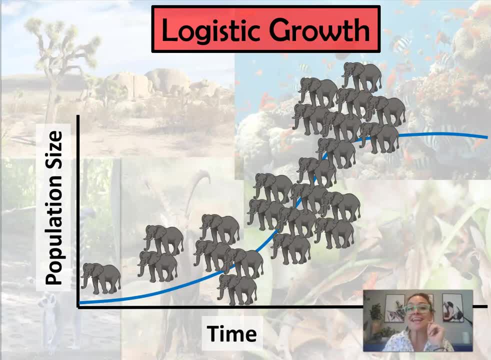 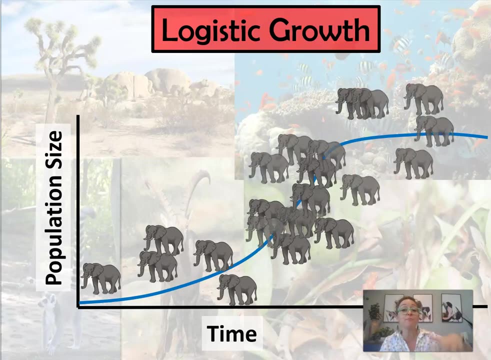 density increased to a very high amount And now there's less resources per individual, which led to more intense competition, which led to not all individuals surviving, And now you have some deaths, but the survivors are going to reproduce, And so then you have births. 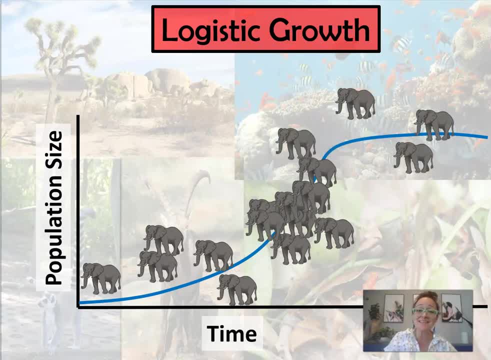 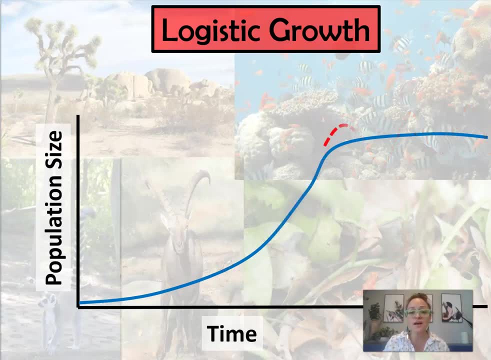 And then if you're above carrying capacity, you're going to have deaths and you find the population is going to fluctuate around the carrying capacity. And so this area here is usually, if you're ever asked to find the carrying capacity, kind of find like the average. if you see it like wiggle a little bit. 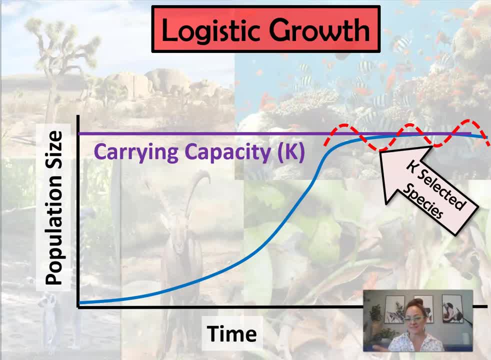 Okay. So the carrying capacity, Okay. So when we talk about species on earth, we can divide them into, like K-selected species or R-selected species, which I'll have a whole different video on just that topic. Our K-selected species are going to be found living in populations that are pretty much 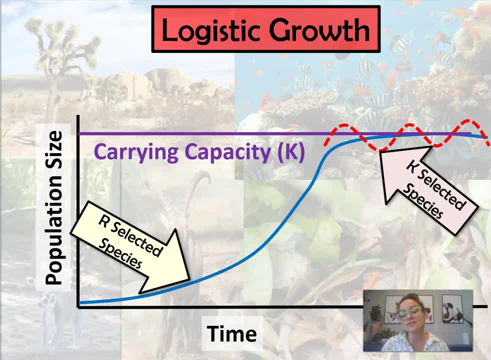 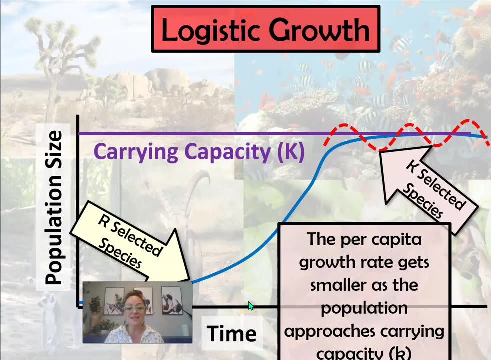 always at or near carrying capacity. And then your R-selected species are going to grow so rapidly that it's like they're experiencing exponential growth, even if it's not forever. Okay, So when we talk about logistic growth, though, The per capita growth rate gets smaller as the population approaches carrying capacity. 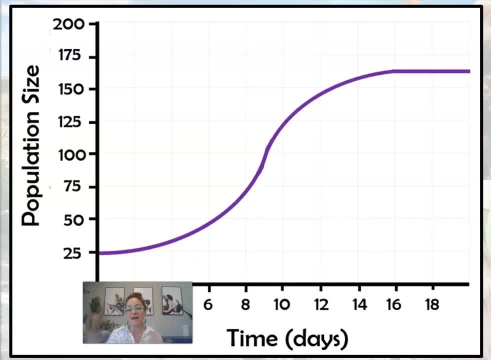 So let's go ahead and talk about how mathematically we can look at logistic growth. So here I have a graph of population over time Now initially. so let's pretend. let's pretend that there was a forest fire And so the forest was cleared, and now we have this open soil and new seeds, land on the soil. 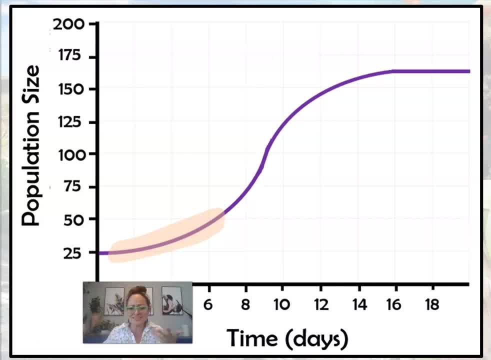 And they start, the rain happens, and it starts to germinate and they're like: Ooh, this is like unlimited resources. Ooh, they start to grow And so you start to have a growth rate begins to increase And then, right at this purple area, there's like a high growth rate. 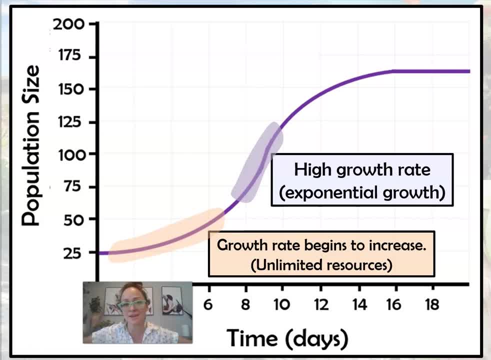 This population is like thriving in this open forest, because it was like there was unlimited space, unlimited sunshine, it's raining, there's unlimited water and growth is good. So if I compare this orange to this purple region R, The rate of growth is going to be higher. in that purple area is a very pretty like steep. 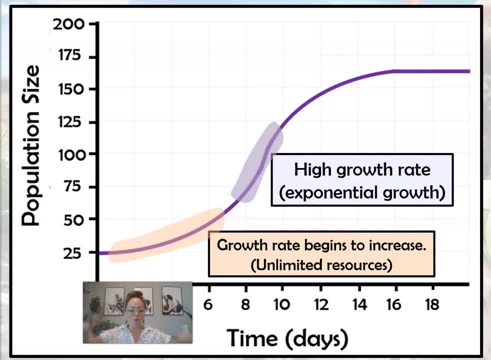 rate of growth. However, as the plants begin to take hold within that forest- now any new seedlings that start to germinate- there's already existing plants. So competition for space is going to become intense and the growth rate is going to slow. 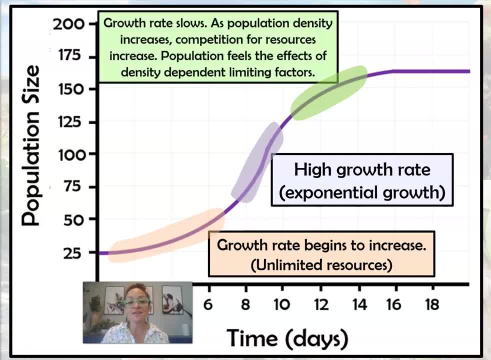 as the population density increases, The population begins to feel the effects Of those density dependent limiting factors and your rate of growth is going to decrease. Now, eventually, you get to a point, possibly, where the population, birth rate and death rate are equal, And so this at carrying capacity, the rate of growth is zero. 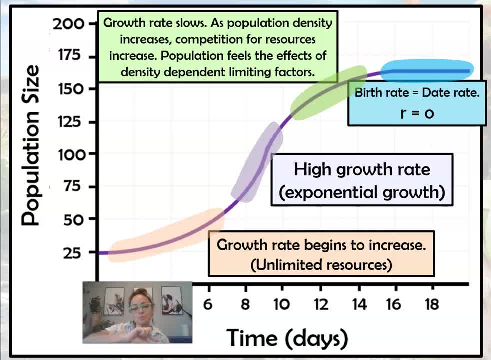 The population is stable. So we can see, as we go through logistic growth, the rates of growth is going to change as the population density. The rate of growth is going to change as the population density also changes and we take into account the amount of available resources, density, dependent limiting factors such as 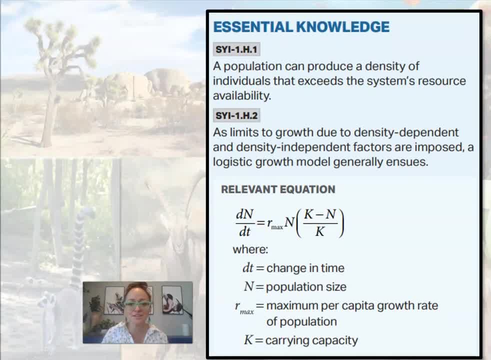 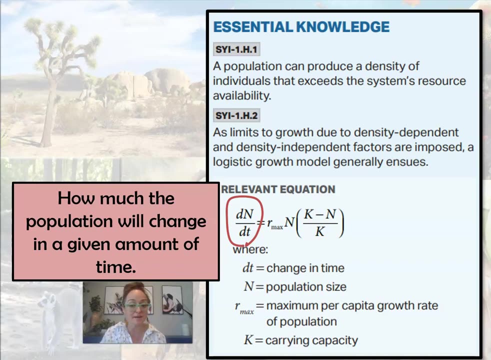 predators and disease, et cetera. competition. So there is a formula, though that goes with taking into account carrying capacity. So here I like to think about this left hand side as like: how much will the population change in a given amount of time? 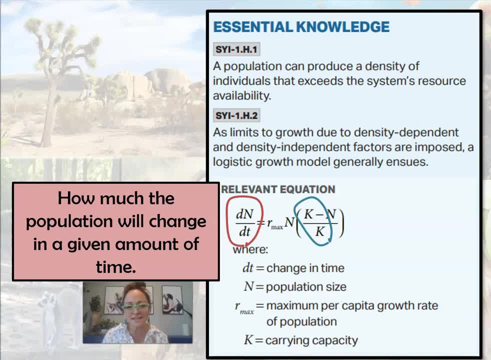 So we have our R max still, But we also now take into account yo. there is a carrying capacity. It's going to get intense As the population gets closer and closer to that carrying capacity. it's going to be harder and harder to survive. 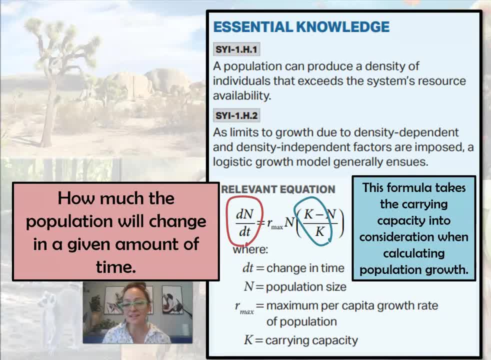 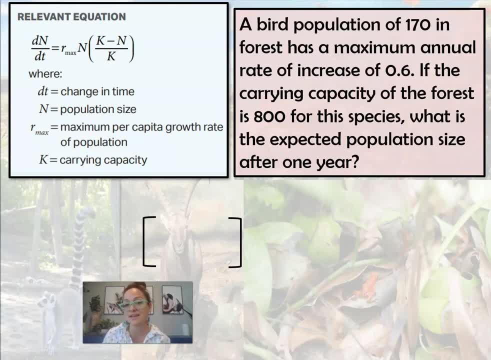 And that's why we include K in this formula. So let's go ahead and see just one example. So if we have a bird population of 170 in a forest and the forest has a maximum annual rate of increase of 0.6.. 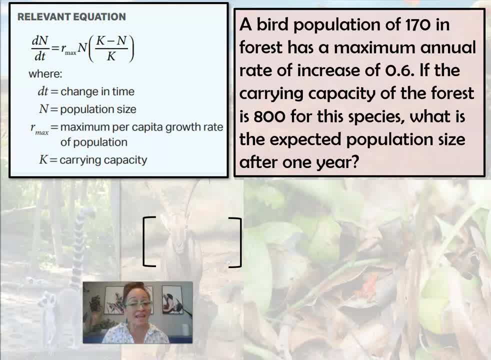 So that's our R value. If the carrying capacity of the forest is 800 for this species, what is the expected population size after one year? Okay, So here we have our, our, our max, our rate of increase is 0.6.. 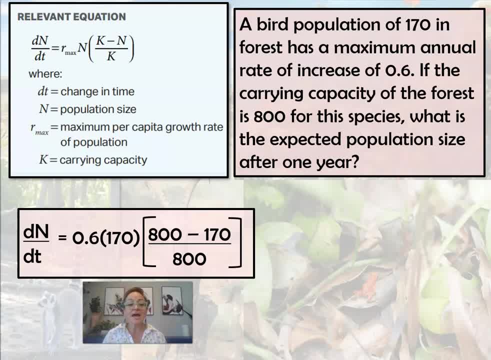 Now our existing right now population is 170.. And then in the brackets we see we'll what will happen as the population is increasing at 0.6 R, As it gets larger and larger it's going to increase. So that's our R value.